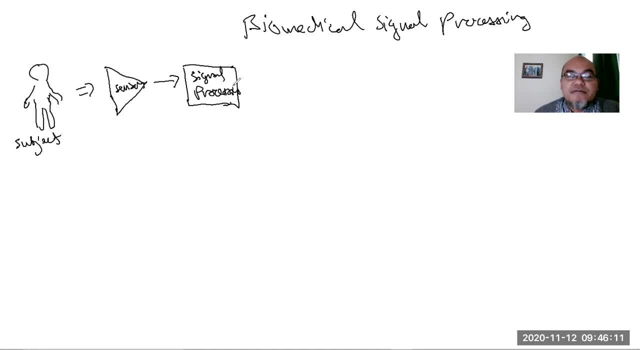 processing before, before the signal can be displayed. so here is signal display. signal display here is further divided into: among others: it could be displayed, yeah, as a monitor, for example. graphic display could also be recorded. previously it was recorded usually in paper as charts, but nowadays with computers, you record. 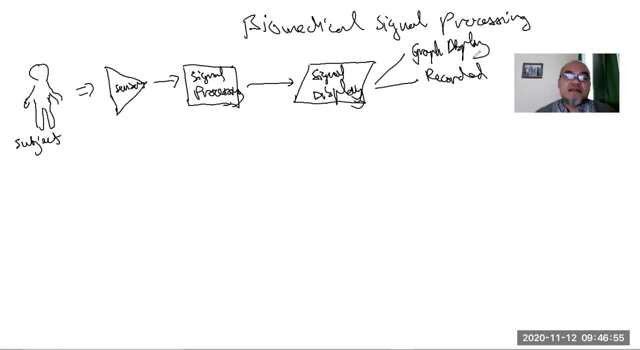 the numerical data, so that then you can easily plot it as a graph in any computers recorded, but also then could be transmitted, especially with internet, with telecommunications, with the advanced in telecommunication technology on the internet now the signal is able to be transmitted across the entire wide world. 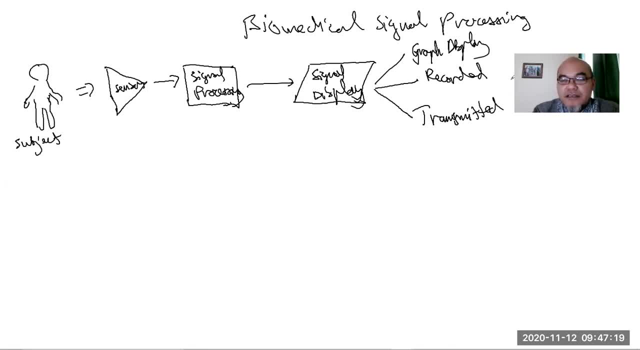 covert means centralced system. the signal is able to be transmitted to anywhere around the world and Поэтому k therapists and aunties, and don't worry, you have access to these E Internet na in location in the Havens, which is my doctor's area called the Heavens Bay. 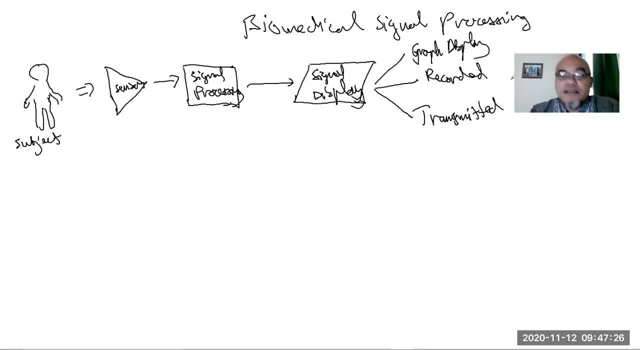 internet technology. now the signal can be easily transmitted to anywhere around the world, so the physician or the doctors, the specialists, do not need to be in the place of the patients. although it is not yet widely used yet this technology, but it is already possible, and later, with the advent of 5g technology, in the future, in the near future. not only that, the physician, some 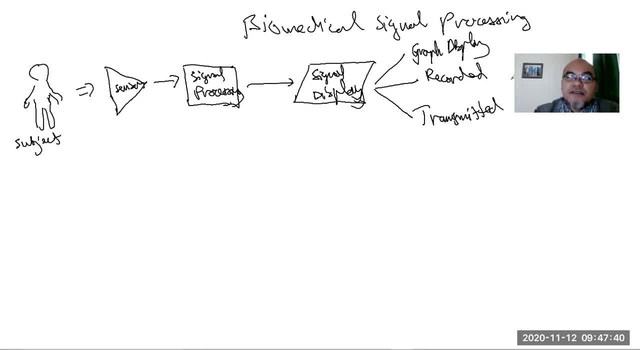 veteran� mano Напрotsky, where may many directors were able to use it- the physician- not only the physician, the doctors or the specialist- can get the data and read the data after it has been done, but the physician or the doctors can also read the data in real time and also possibly. 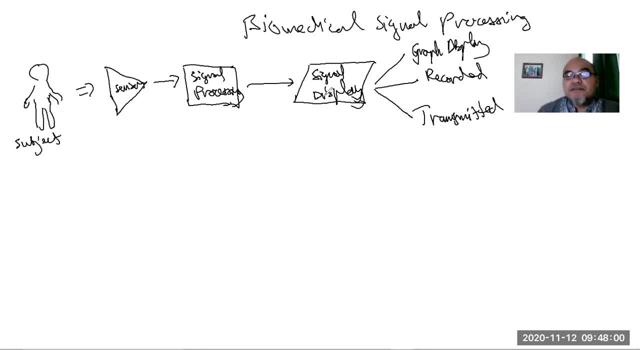 do the therapy also in real time. It will be something in the future that also this will involve, for example, in future surgery. This is already in therapeutic case. Well, this mostly is still in diagnostic part. Even now, the diagnostic part has not been done completely online or in real time. 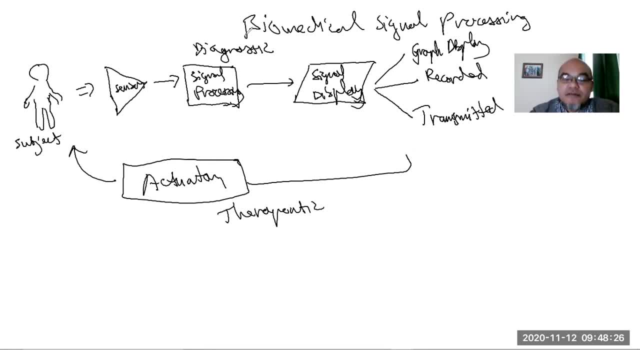 Mostly still, in most of the most of the clinics, even hospitals, they do it still offline. But already data are being recorded. Previously, even in 20 years ago, mostly are still in papers, in chart paper, And the doctors have to, or the patient or the nurse have to, bring this printed charts into the physician, into the specialist, to get their information being interpreted. 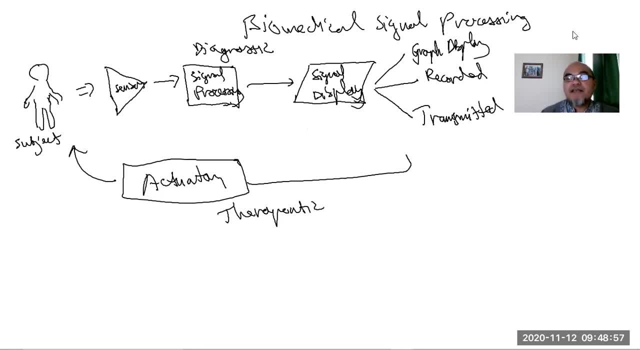 And now, even with the advent of AI artificial intelligence, some of this can also be recognition, signal recognition. And now even with the advent of AI artificial intelligence, some of this can also be recognition, signal recognition, Recognition and interpretation. 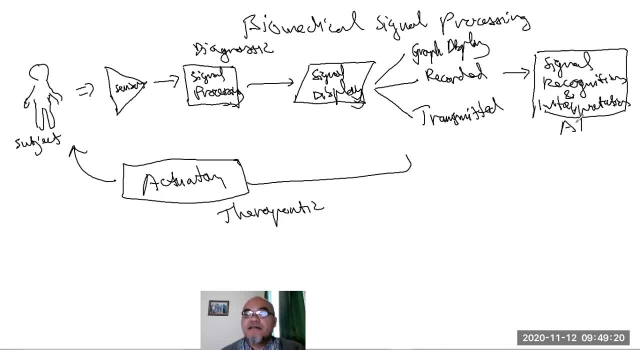 Interpretation. So especially using AI. In my time we actually we already learned about artificial intelligence And but we haven't really applied it in actual healthcare. We just learn it for the sake of knowledge or for the sake of science. 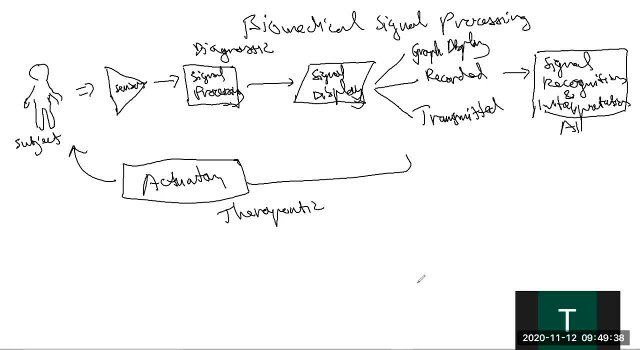 But today it is almost there, The technology are there. So now people are developing this technology to be able to interpret the information, the signal automatically. So, for example, like if you know what Paolia is is doing for his research he is doing, he is developing artificial intelligence algorithm, machine learning algorithm. 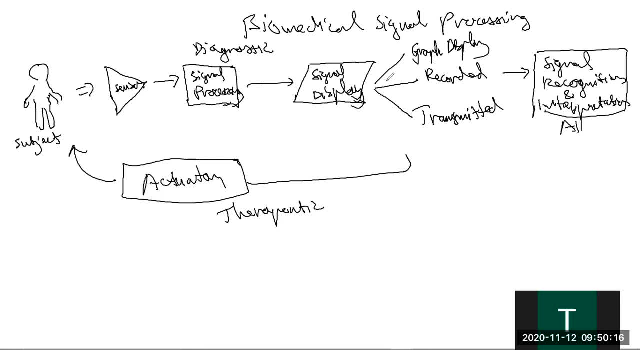 that can classify ECG signal autonomously- actually without the help of cardiologists- and then interpret it, whether it is whether the person is healthy or not healthy. If not healthy, what kind of diseases he or she has? Is it arrhythmia? 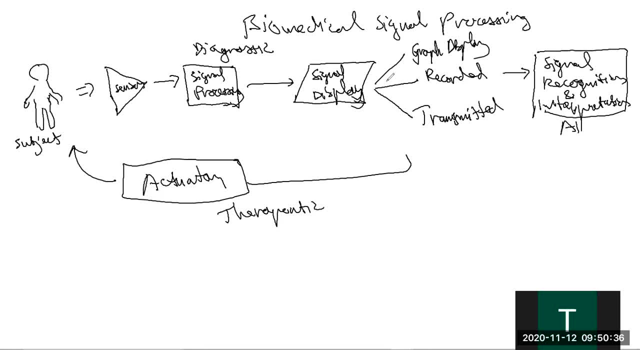 Is it dysrhythmia, Tachycardia, for example, and many other heart related diseases. So this can now even be replaced by an automatic system, even though there is still some resistance from the doctors, The cardiologists. they do not yet, they are not yet really want that. 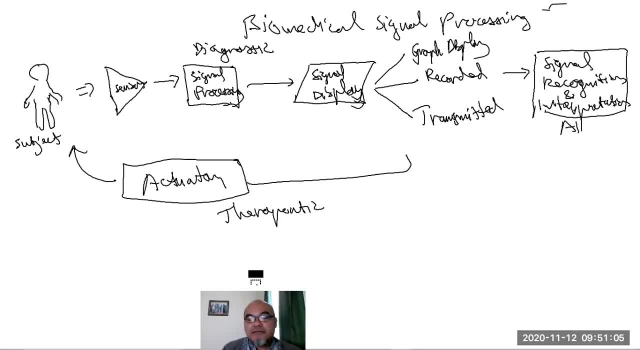 their role is being replaced by a system, by a machine system, by a computer. But, like it or not, actually there is a need for that Because if we see our condition in developing countries, in Indonesia we have remote regions. Our geography is, we are an archipelagic country with islands spread in thousands of kilometers away. 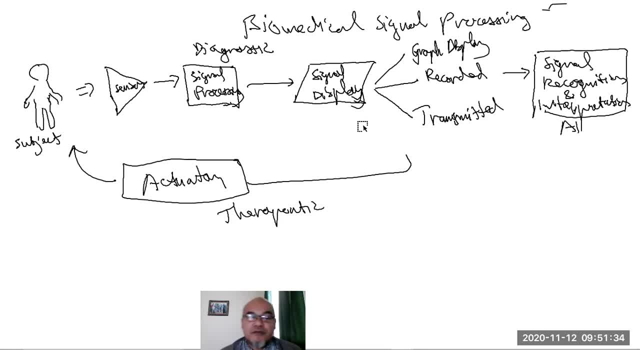 So, and most of the specialists, most of the good doctors, live or reside in big cities, in Jakarta, in Surabaya, in Medan, like that. Well, in remote regions, even in West Java, for example, in the remote region in Tasikmalaya, Sukabumi, 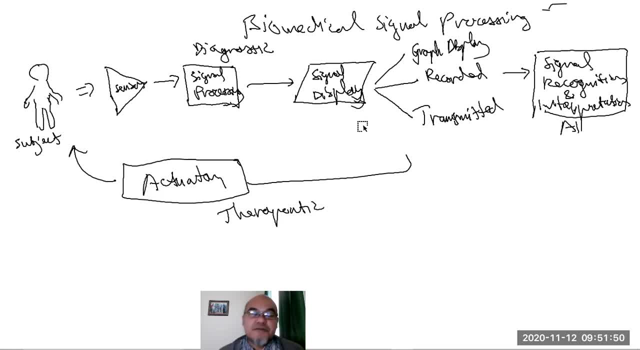 in the villages you cannot. it's very difficult for you to find good specialists. So how can we make a more distributed, or evenly distributed, healthcare service? One of that is by exploiting telecommunication technology and information technology using AI, artificial intelligence. 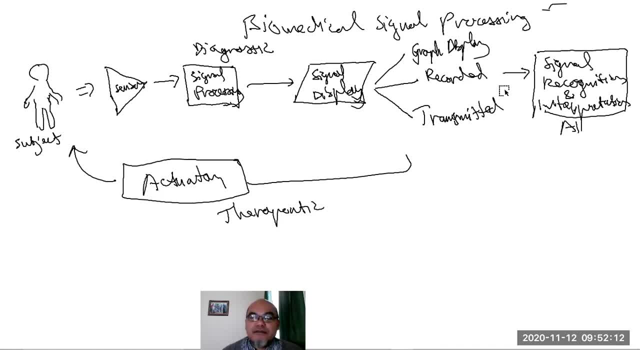 So there is more and more movement towards not only to display the graph, the data from instrumentation, not only to record the data, not only to transmit the data for telemedicine, but also to automatically recognize the data, to interpret the data and give already ready information for either the physician or the patient himself or herself. 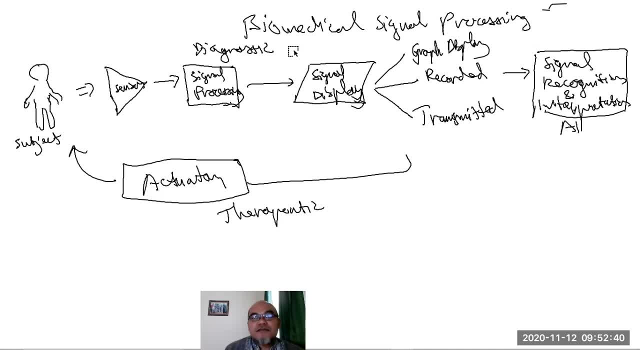 And in the near future, this even goes towards therapeutic. So, as I mentioned, we are moving towards this direction with the advent of 5G technology. In 5G technology, the speed of telecommunication will get, will be getting more enhanced. 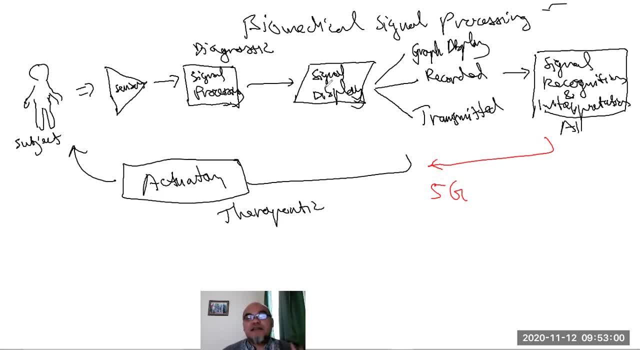 Such that there is no latency anymore. Latency here meant the delay in telecommunication. Currently, if even, for example, if you do telecommunication at the teleconference using Zoom or using video, sometimes you see some delay between the voice and the image. 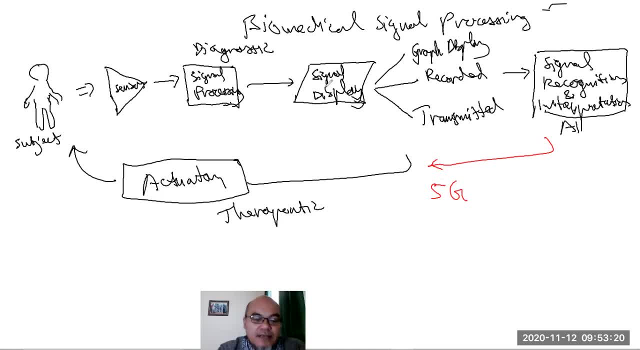 In the future, this delay will be less and less, even more, even less and less. So this is very important when you want to conduct, for example, telemedicine, So the doctor, the surgeon, might reside in Jakarta, The patient with the nurse may be somewhere in Papua, for example. 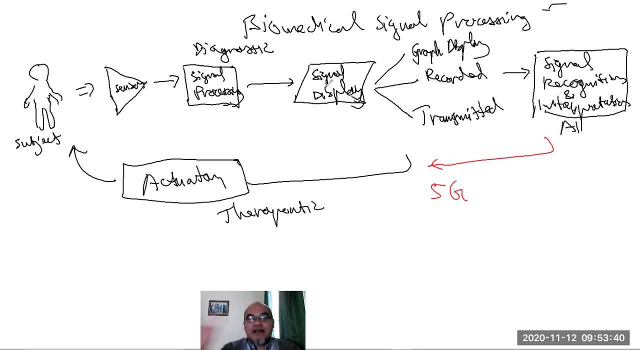 And then the doctor see a real time image, video imaging- from the patient in Papua and then immediately operate some machine in Jakarta to operate, for example, the heart or the stomach of the patient somewhere there in Papua in real time. We thought the 5G technology. this is not yet possible. 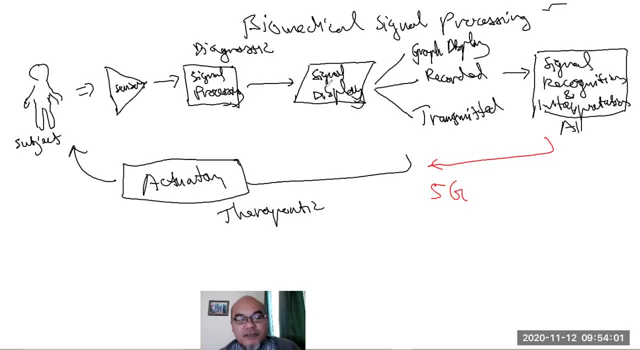 The current telecommunication network which we have in Indonesia, 4G- it is not yet possible because there is still this latency between the person operating and the actual activation by the actuator at the place where it needs, where it needs. So, but for example, in China, they have already used this 5G technology. 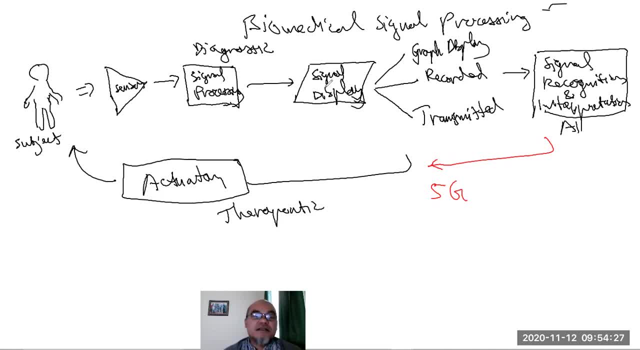 Even though not yet in the health care sector, they use it in the industrial sector to operate, for example, big machinery tractors, forklift, especially during the pandemic, And the operators just conduct the operation in some special room near their house. 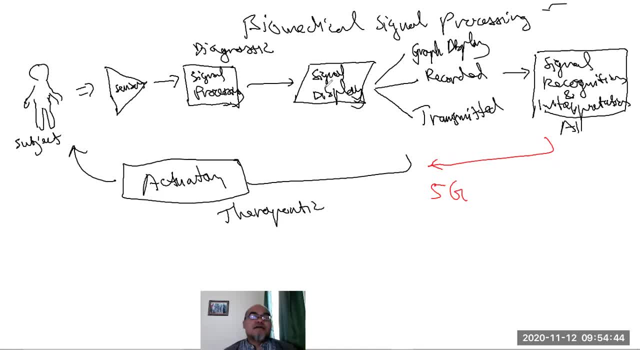 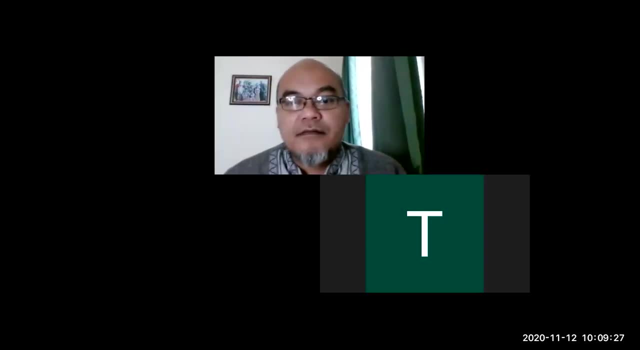 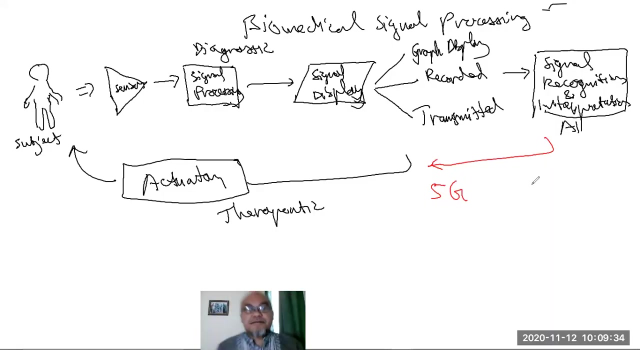 And then the machine is on the field. So this is made possible using the 5G technology. OK, so let's have a break for a while. Sorry for the delay today, because I have some meeting, So we go back to this. 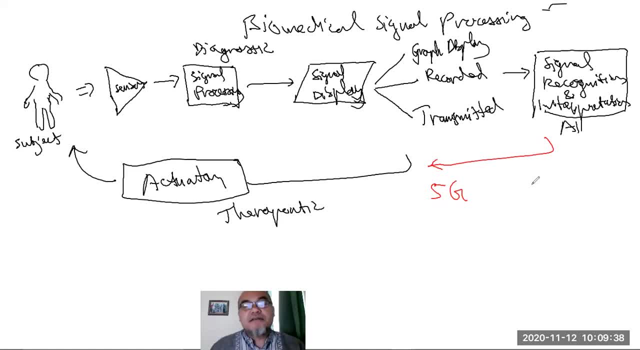 Now what usually when we speak about signal here? So signal here is what? the video that you have just seen, what you have just seen in the YouTube. There are many types of signal. Of course, one is one value signal. This is like body temperature or something like that. 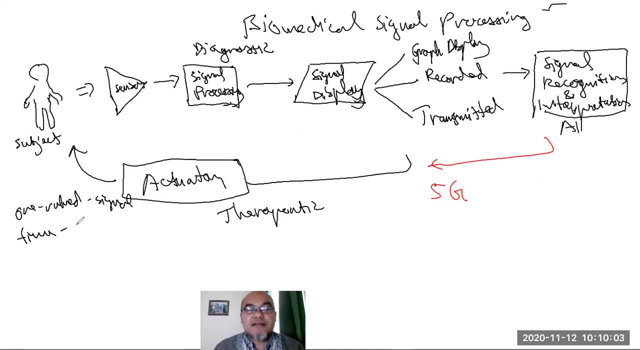 But there is also time dependent signal And many of our biosignal, biomedical signal, are time dependent signal. So in this case, that they are a function of time. Let's say, for example, ECG, electrocardiography. This is the signal from our heart. 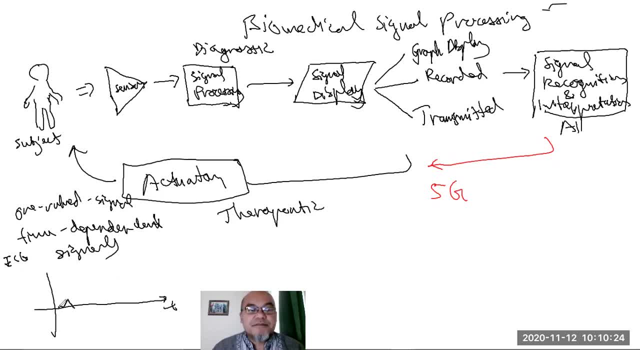 And usually then it looks like this: This is the P and then Q R S T. So this is the P- Q, then the R peak S, then there are small peak T here, Then again another P, Q R S T, etc. 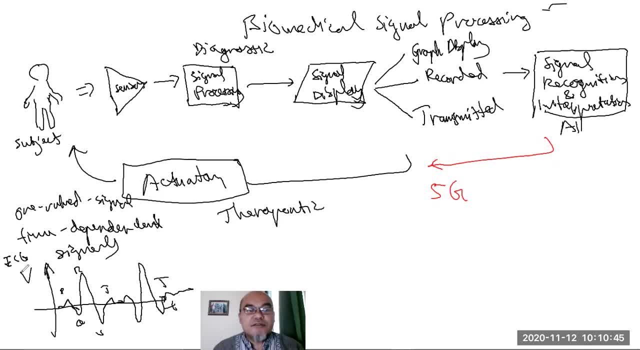 OK, This is usually is voltage, because we are measuring in In in voltage, because the ECG measure the potential between two or three or more of potential difference of places in the body, mostly near the vicinity of the heart. So this is the time domain signal. 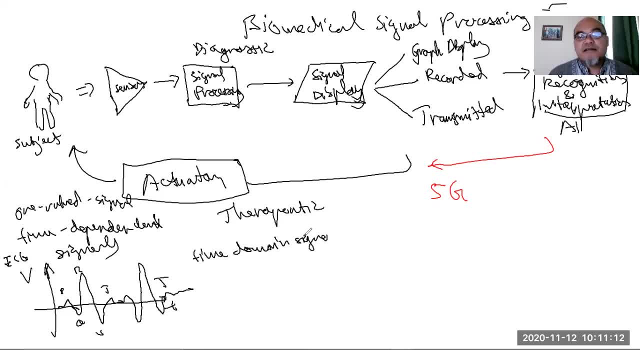 So in time domain signal, mostly, we express a signal in three parameters. in three parameters. What are they? They are voltage or the amplitude. the amplitude, Then we have the frequency of the signal, Then we have the phase of the signal. So this is, if you know from mathematics, 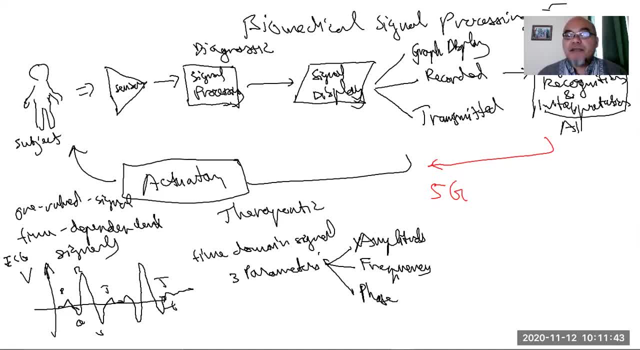 Yeah, Usually we express time domain signal in terms of sinusoidal signal. So if you have only one single sinusoid, for example like this: Yeah, this is a sinusoidal signal as a function of time, Let's say this is a function of voltage. 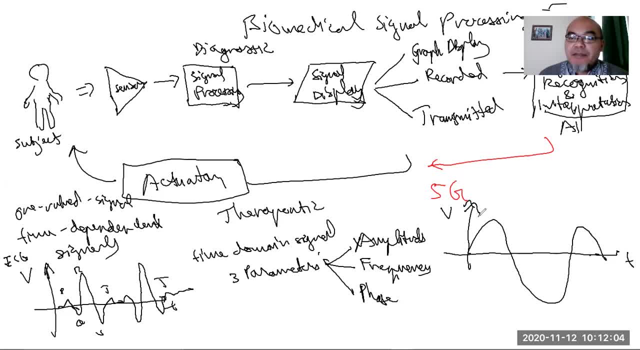 OK then the amplitude is the peak value, the value of the peak. This is the amplitude. Sometimes we want also to see peak to peak value. So amplitude, peak to peak, So here. So if only just amplitude, usually it's from the zero level to this one. 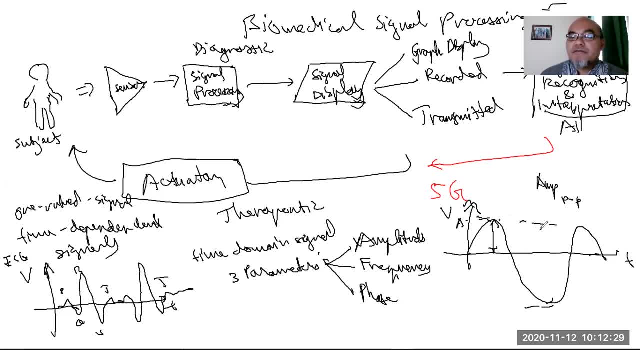 But if it were peak to peak, usually from the positive peak until the negative peak, This is amplitude, peak to peak. The frequency is the second. The second parameter is the frequency. It indicates, or it shows how many times that signal Repeat itself. every every second. 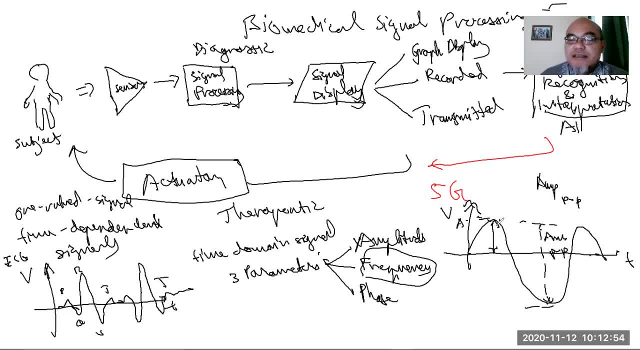 So, for example, if you have a sinusoid like this, right It repeats itself from, for example, this is repeating itself, or this peak is repeating itself here. So, basically, the period is when it forms a single wave, a single full wave. 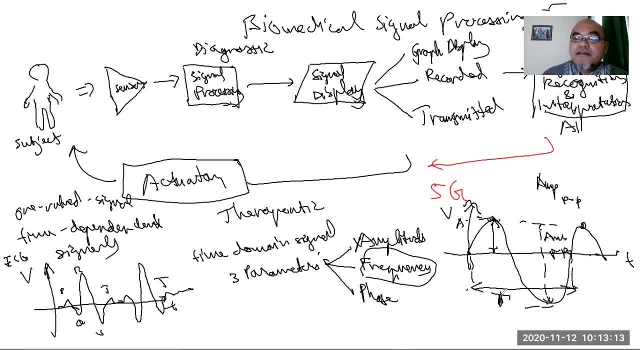 This is what we call a period, right, How many seconds? So then the frequency can be defined as the inverse of the period, one over T. So, for example, if we have a sinusoidal signal whose period is one millisecond, It means that the signal repeats itself every one millisecond. 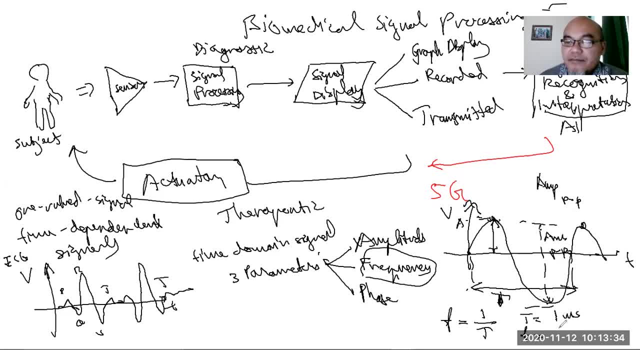 So the frequency will be: how many? Anyone, No one. Is everyone still Alive here Sleeping? Hello, Is that one millisecond, sir? Yes, if the period is one. Yes, the frequency will be One thousand. Yes, so the frequency will be one over T. 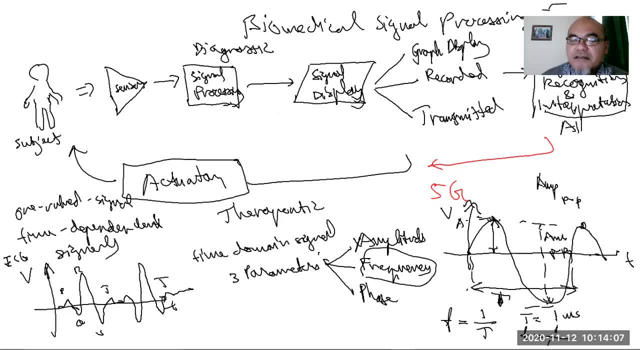 Right One over one million. one millisecond is 10 to the power of minus three right, So this will be one thousand. Yes, So this is the second parameter. The third parameter is what we call as phase. Phase is how much time it is lagging or leading. 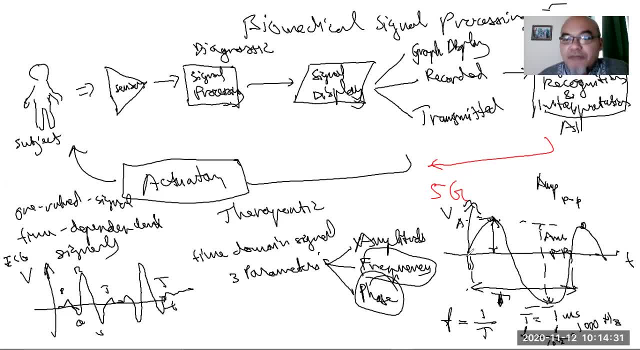 So, for example, if we have another wave, that when the T equal to zero is already in its peak here, So we know that it is leading by 45. Sorry, by 90 degrees, right? Or by? usually we express the phase in radian by pi over two radian. 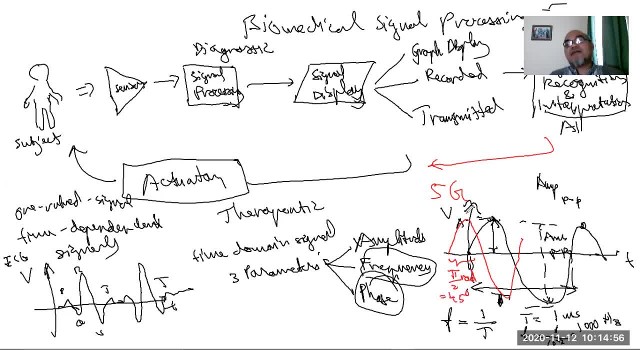 So pi over two radian equals to 45 degrees, Because at 90 degrees 90 degrees, 90 degrees. So because at T equals zero, in normal sinusoidal it is supposed to be The sine zero is zero right. 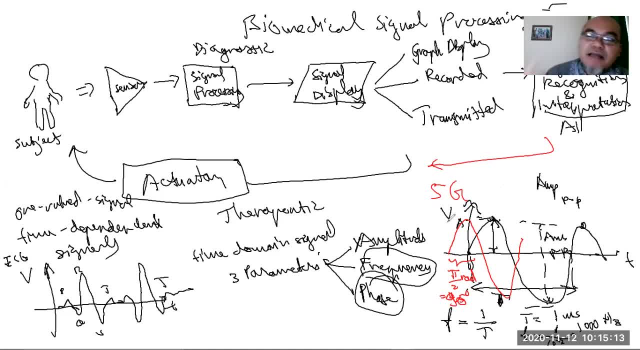 So this red wave by time equals zero, is already sine 90 degrees. 90 degrees is one. So we can express then the black wavelength as, for example: is this one Y equal, Let's say the peak is A Sine. 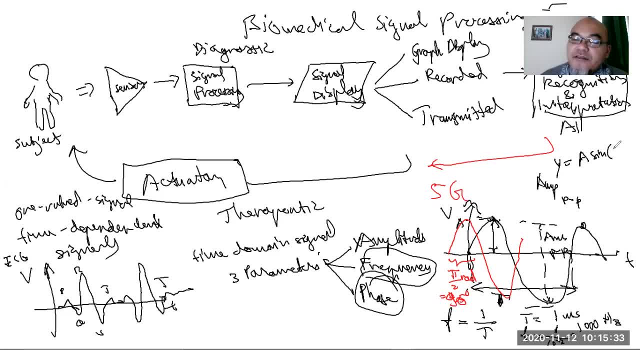 The frequency is one thousand hertz, So usually we express the sin omega T, where omega is the radian frequency. Radian frequency, or cyclic frequency, is defined as two times pi times the frequency. So in radian frequency it's not anymore cycle per second, but instead it is radian. 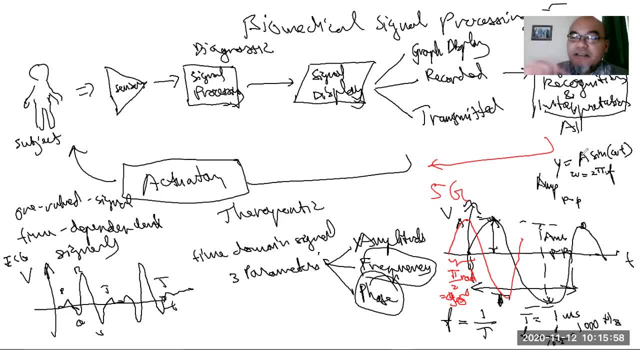 How many radian per second. So let's say, if it is one hertz, one cycle per second, it means every second it is two pi Right. Every second is two pi radian. So the omega will be two pi times one. 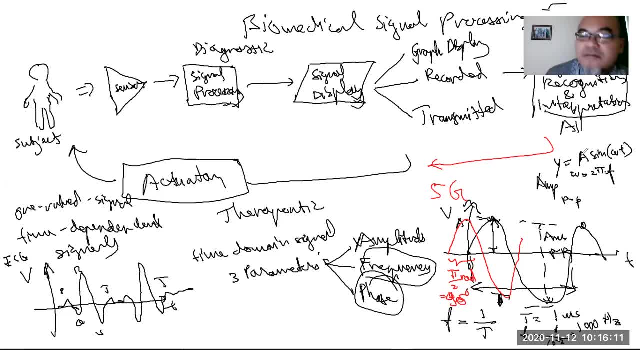 Two pi per second, Two times pi, 6.28 radian per second. So in the case of one thousand hertz frequency, then the black wave here is Y. equals to A sine two pi. two thousand pi T. Sorry, T times T. 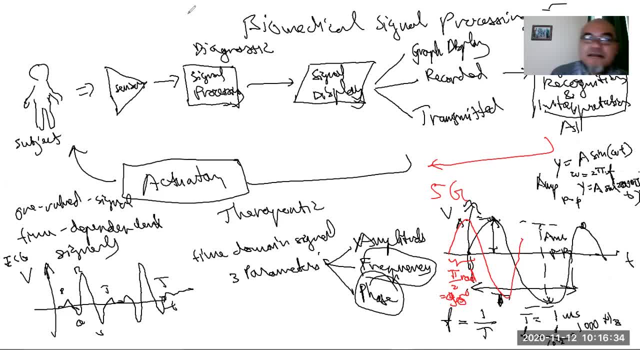 Okay. Well, the red one, the red wave here, will be: Y equals to Y dash. Let's say Y dash. Okay, The amplitude is the same. Yeah, Sine, Two thousand pi T, And then plus pi over two. 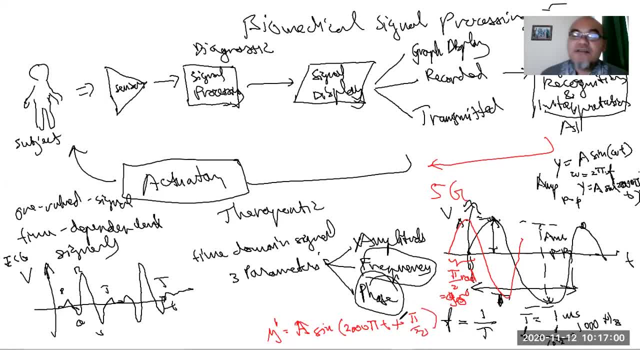 So this is the phase. So, because at T equals zero, it already has a phase of pi over two or 90 degree. That's why the value of the red one is One. Yeah, Not zero anymore. Okay, This is safe. 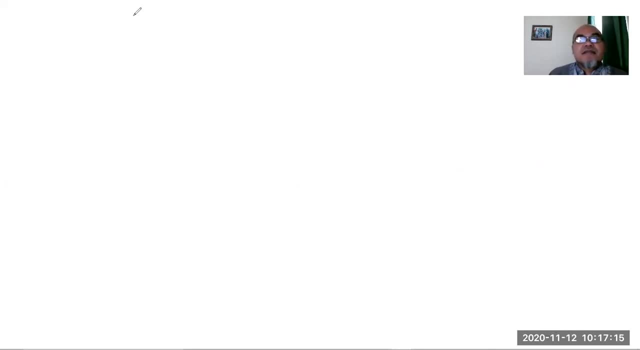 That's now clear, Okay. So sometimes or not, sometimes many times the signal like ECG, but we have seen what I have just drawn: The signal can have multiple frequency, multiple frequency, So the signal can consist of not only a single sinusoid. 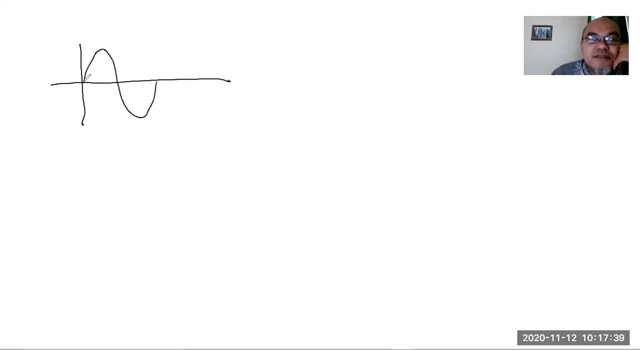 But in second is of multiple sinusoid like this, And then you have with having a frequency of F1, let's say, then we have another, Another signal consistent, consisting of frequency equals to two F1. So this it means it will have, the amplitude is the same. 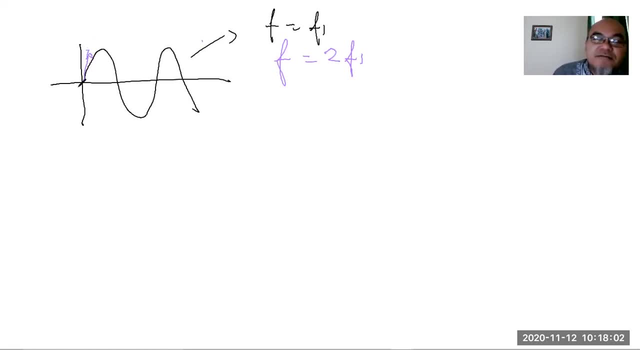 Let's say the face is zero, So it's having the same face at the equals zero. So if I, if we draw it, it will be, it will look like this, So something like this. See here. So it is twice. 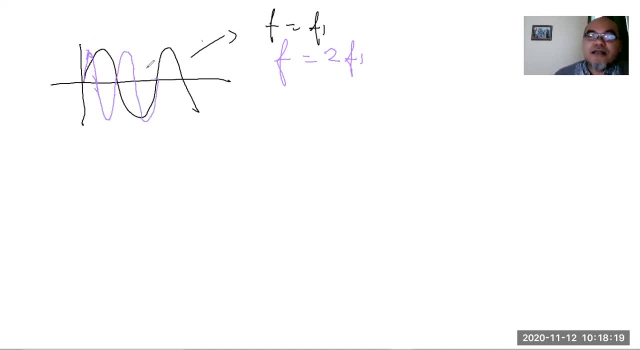 Two Quicker, Yeah, Or two cycles more than The first Signal. Then the overall Signal We look As Will be: Y Equals to A Sine Two by F1. This is, it is F2.. 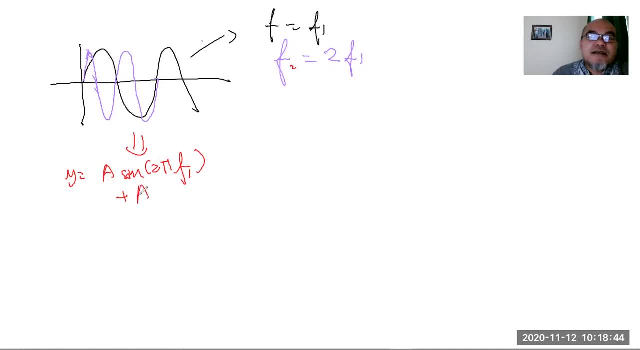 Plus A sin, Two by F2.. Okay, So this will look like something like this, Something like that. So it, because it has, or it has to, Two Frequency. So, And we can add more, Not only two frequency, but even more than two frequency. 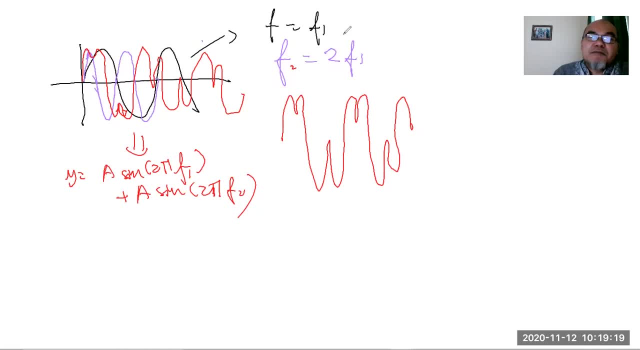 So when, When the frequency is A multiplication of a base frequency, the next frequency. So, for example, we can have F3.. Equals to three F1.. We may also have F4.. Equals to four F1.. Yeah, So when we draw the 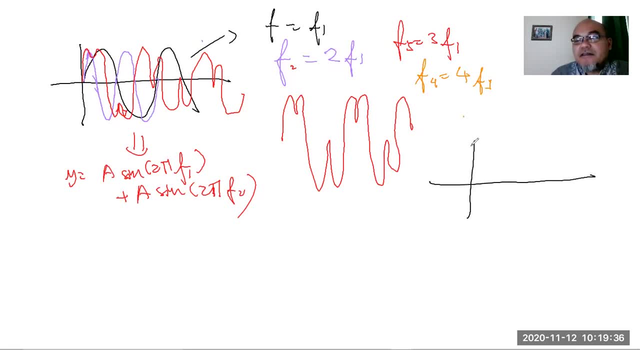 Signal, then we will. So we have This addition, Summation of all this frequency And this is what we call as harmonics of the base frequency. So the base, This is called as the base frequency and the other frequency are called as the harmonics. 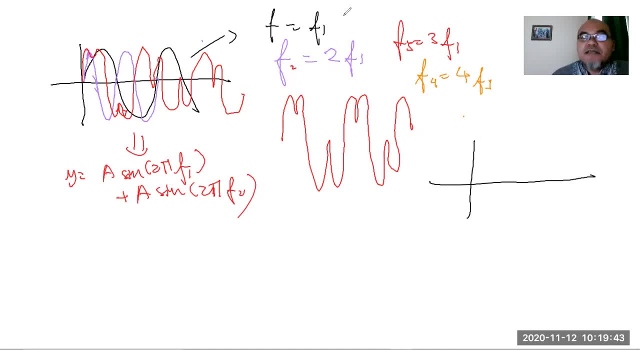 Of the base frequency. So the two will be the second harmonics. We call it Three will be That harmonics. The Four, F1. Will be called as the four, Fourth harmonics. Okay, So So. 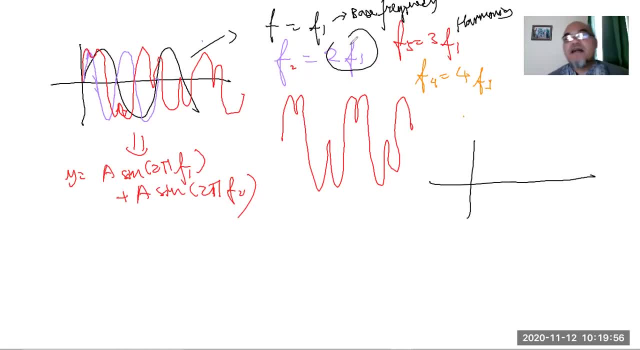 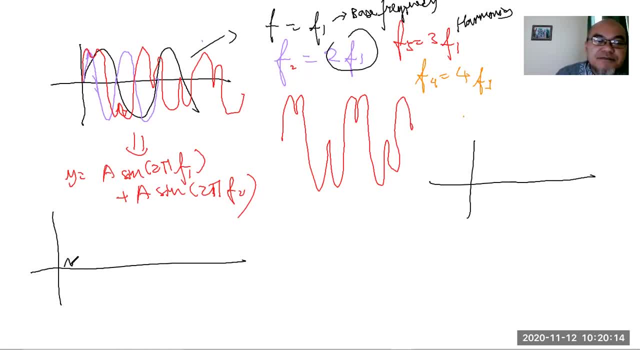 I think this one will, After Next, Then be the second For each signal. So Do you know that? I mean, yeah, I, Exactly, It's the same, but it's it's very, very Right. 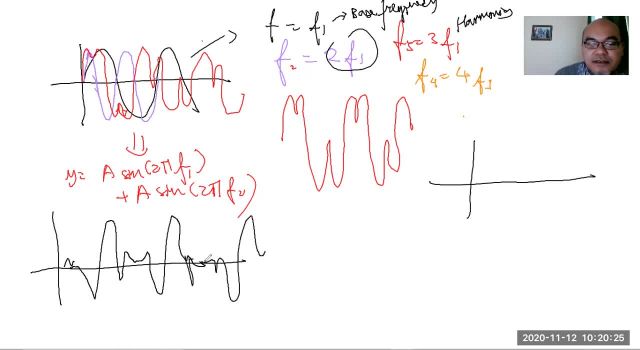 Let the signal- There is different scale of that- is also Communican emission, So that this one Is going to equalize Per binding frequency, So Now contain much more frequency than just one single frequency. First, it is not sinusoidal, but we know it is periodic. 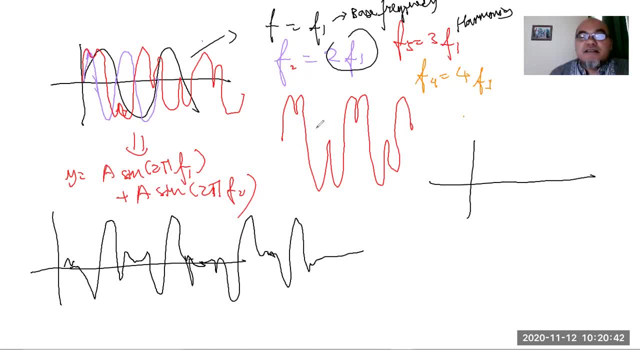 Then we need to do what we call as frequency analysis. So this is from time domain, this is t time domain. signal voltage as a function of frequency. We would like to change it into frequency domain Signal. so we want to know the frequency component of this signal. 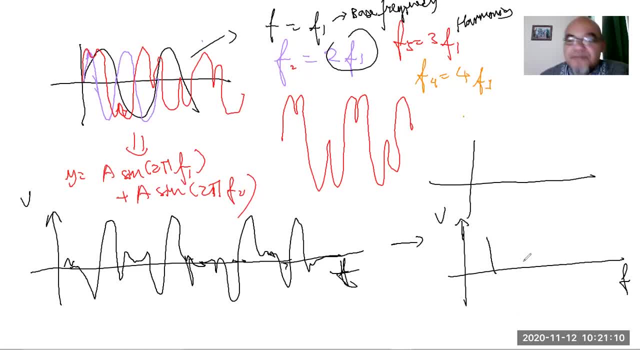 What is it made of? Is it made just from a single frequency? If it is like this, if it is F1, F2, F2, which is two times F1, this is the harmonics. But a signal like ECG, which is more irregular, consists of more than just the harmonics. 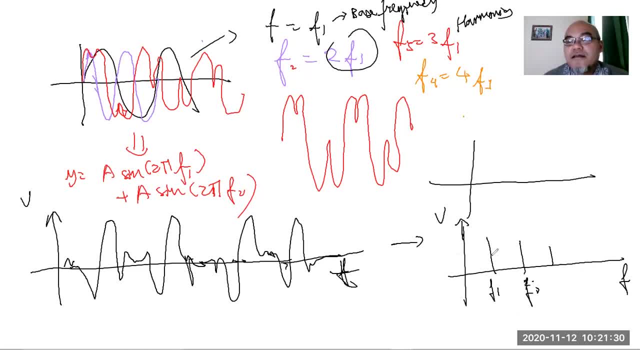 the base frequency and harmonics, which contains also other signals, So this can. so usually in the case of, in the case of ECG, the bandwidth is until 100 hertz. Yeah, about 100 hertz, the bandwidth. we call it as the bandwidth. 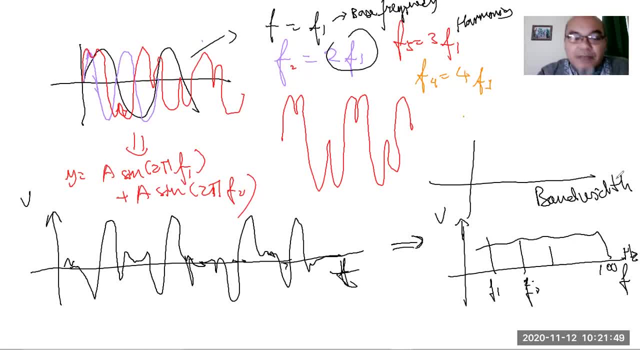 The bandwidth is the signal having frequency, the range of the frequency of the signal that form a time domain signal. In the case of ECG, it will be about 100 hertz. Okay, In the case of EEG- electroencephalography brain- the bandwidth could be up to 1000 hertz. 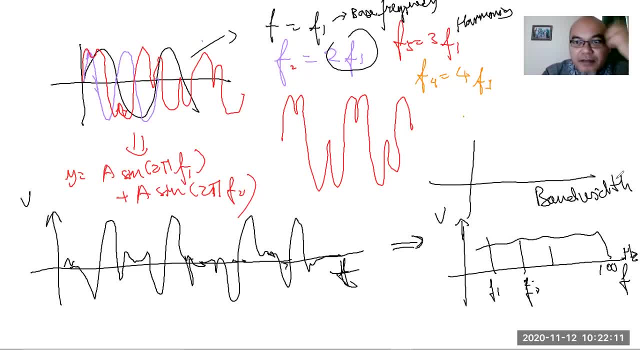 Muscles EMG can be around tens of hertz, several tens, yes, several tens of hertz. Okay, The the tools to transform from time domain signal into frequency domain signal is usually called as Fourier transform. okay, Fourier transform. 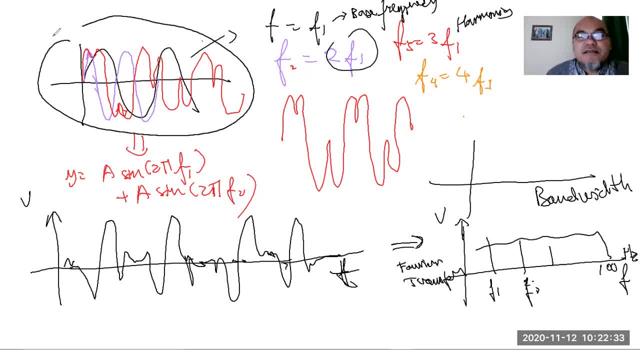 Okay, If the signal is still simple like this- yeah, consists of frequencies which are basically the harmonics of the base frequency- then we can use Fourier series to express it, because the signal is still periodic. But when the signal already contains a lot of a lot of non-periodic component, then 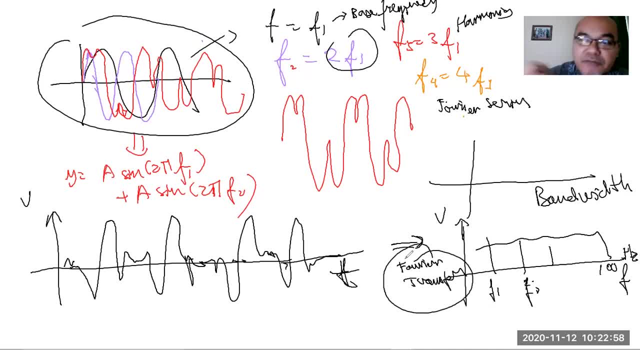 we have to use Fourier transform, And when we we do it in computer, the algorithm is usually called as fast Fourier transform, Okay FFT. This is the, the algorithm used in computer usually to convert time domain signal into frequency domain signal. 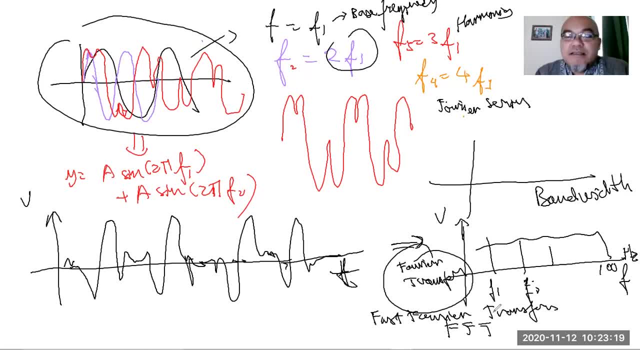 Okay, And why? why do we need to analyze a signal into the frequency domain? Sometimes the not sometimes, yeah, many times the signal we that we obtain from our, our frequency domain, Sometimes the signal we that we obtain from our instrumentation, from our, our, our amplifier? 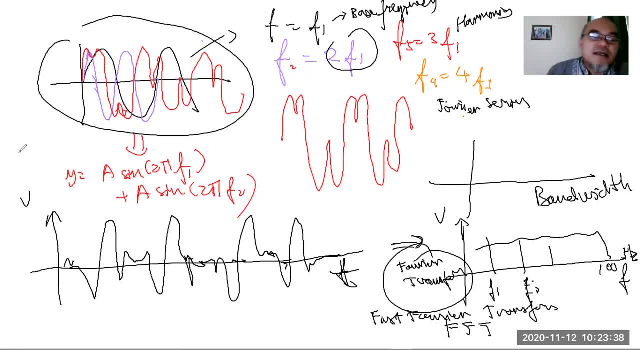 and then our sensor, and then we amplify it and then we filter. It's not, it's not smooth, Yeah, Sometimes like this, this is the, this is the ACG signal. for example, is there is a ripple here? Yeah, 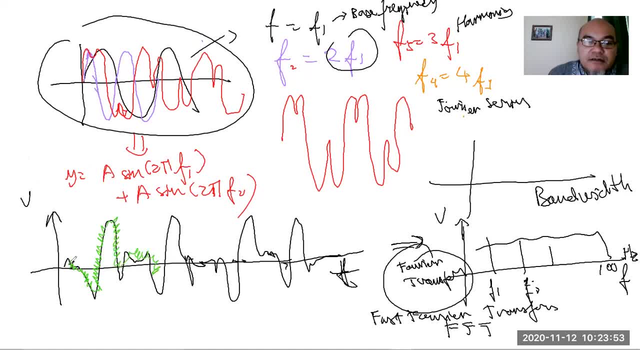 There's a ripple, high, high frequency ripple, Yeah, Overlapping with the original signal. Okay, So when we put this into frequency domain, we will see that, for example, this one will will be from particle frequency, usually from the electricity line 50 Hertz. 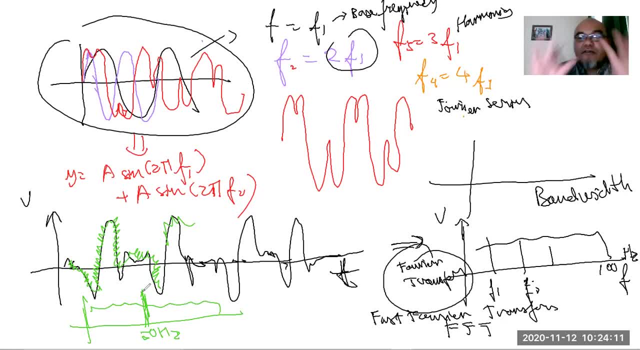 Okay, The other one is like this: the other frequency component, And then we can use filtering- filter to get rid of the signal which we don't want, or the noise and the noise. The noise are signal which we don't want. 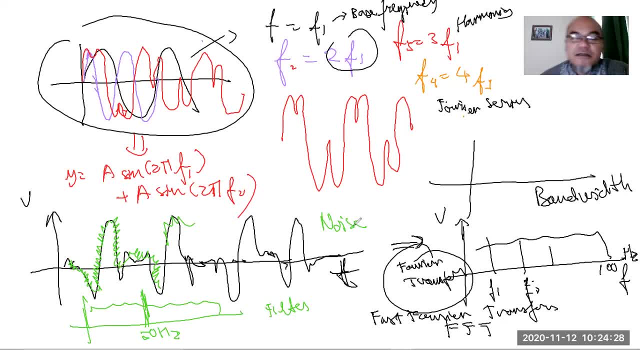 Basically, that comes can either from the instrument itself, can also come from the environment, can also come from the subject, When the subject move. Okay, When the subject move, This ACG signal may be drifted. may be drifted, For example, it become like this: 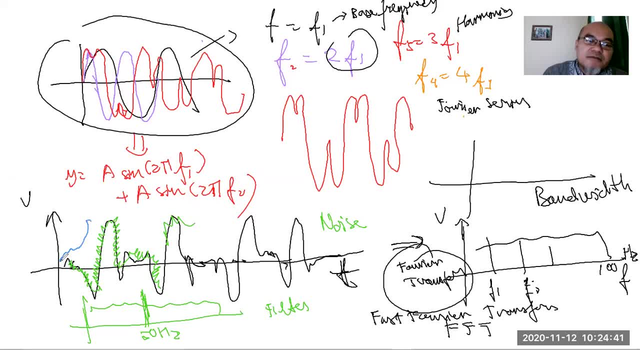 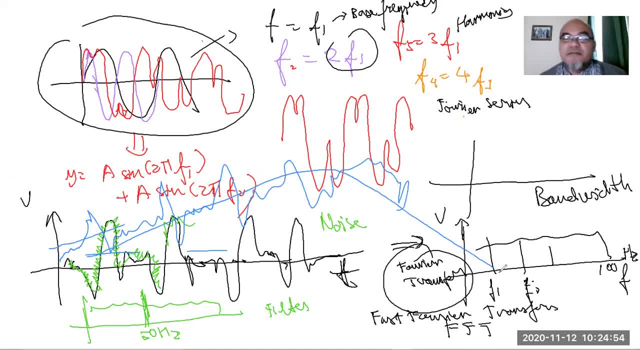 Yeah, Yeah, Yeah, For example of the patient, then this can also be eliminated using filtering. But to be able to do free filtering we have to first transform the time domain signal into frequency domain, So we know the noise, which one is the signal, the original signal from the heart that we 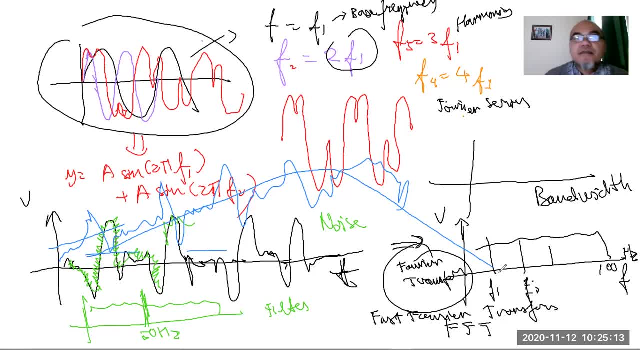 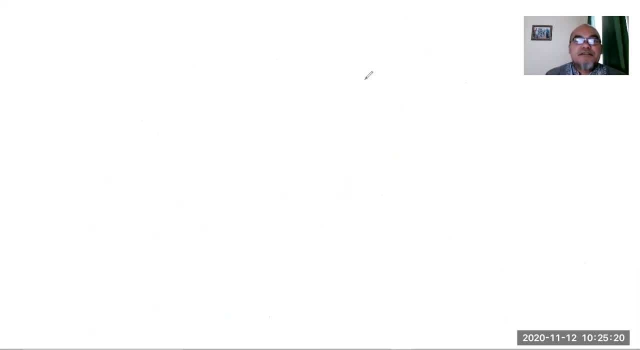 want to measure and which one comes from the noise. Okay, let's say this in the clear. Okay, then another things which we need to know. Usually, What is that? The original signal comes from the sensor and then the amplifier is in the form of analog. 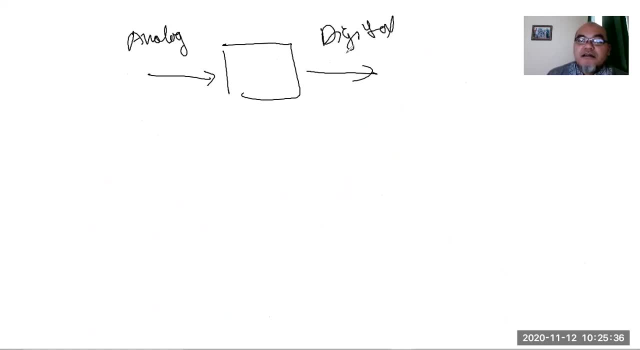 signal, and this one is digital signal that is processed by the computer or recorded, is in the form of digital signal. What is the difference? So, from analog to digital, we need ABC. So, for example, if we have analog, is when we have the signal continuous, like this continuous. 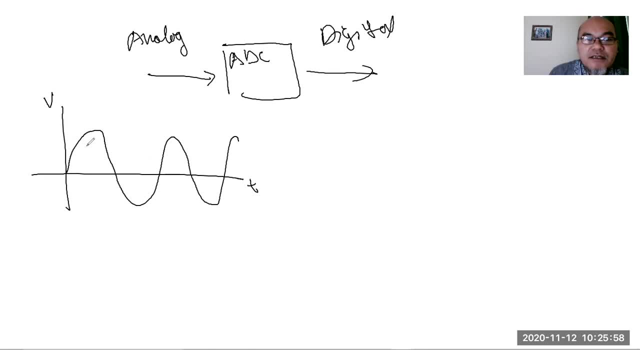 in both time as well as in value. both is in time. it is not disrupted. in value also, it continues from this zero value to, for example, a maximum tenfold, for example. But when it goes to analog digital converter, first it will be sampled and this is what 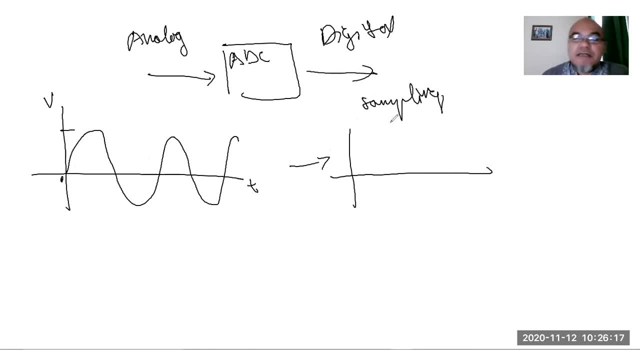 we call a sampling Period, sampling stage. So the sampling means that it will be cut off, cut off at certain place, like this. So we will have instead this signal. this is what this is called as discretized signal, discretization, discretized signal. 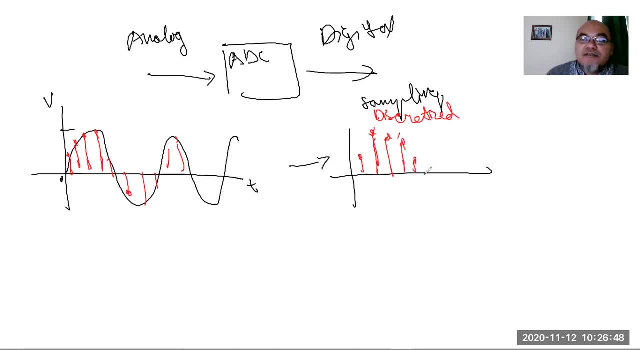 Time. discrete signal Time. discrete signal Time. discrete signal means that it is not continuous anymore. It means it only has value at certain sampling period. This is zero. this is t. this will be 2t, 3t and then n, etc. until nt. 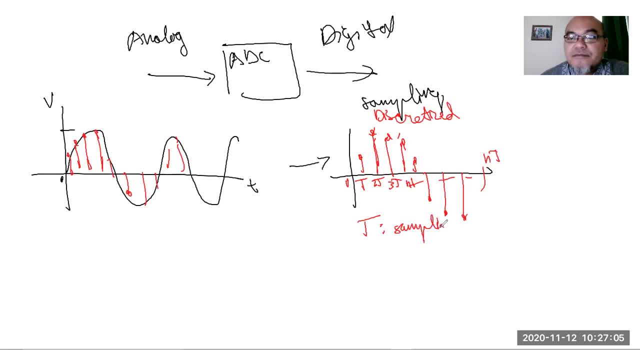 So t. here is the sampling period. So for example, if we have a signal, let's say ECG, we can sample every one millisecond. The one millisecond is the sampling period. It means the sampling frequency. So the sampling frequency will be: this is the sampling period: 1 over ts and the inverse. 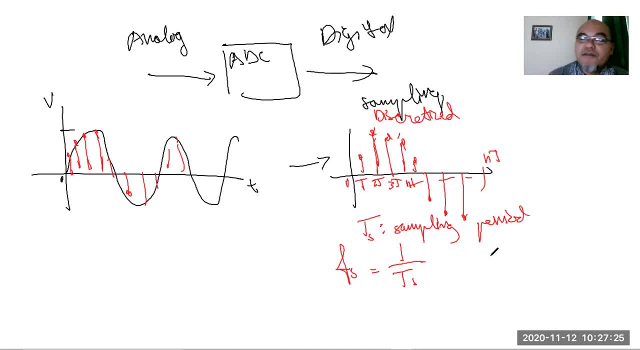 or similar like the formula for period and frequency in the continuous signal. So if we have one millisecond sampling of sampling, period means the sampling frequency will be 1. over 1 millisecond It will be 1,000, not hertz. again, usually we call it as 1,000 sampling per second. 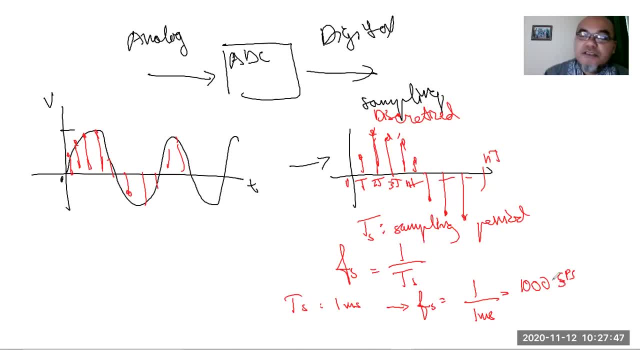 Yeah, we can call it hertz. Mostly in analog-to-digital conversion we call it as one sampling per second or one kilo sampling per second. okay, So, but this is not yet finished. After discretization, what happened in an analog-to-digital converter? is that the signal? 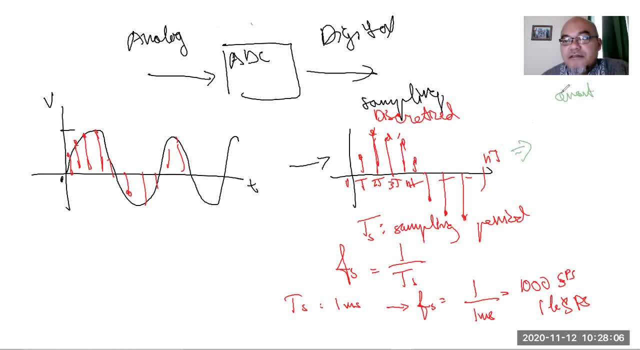 will get quantified quantization. What does it mean with quantization? It means that the signal, the value of the signal, will be quantized Like this. So, for example, depending on how many bits you have. So, for example, let's say you have seven, a value of seven, right? 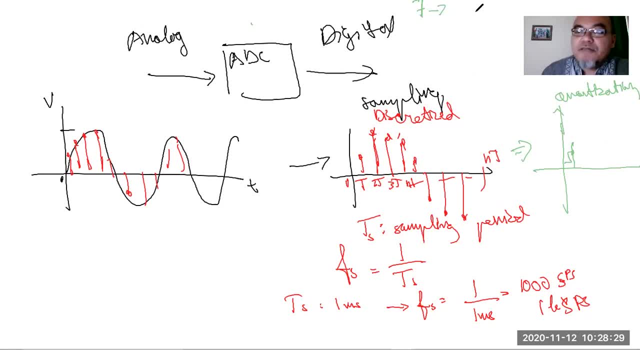 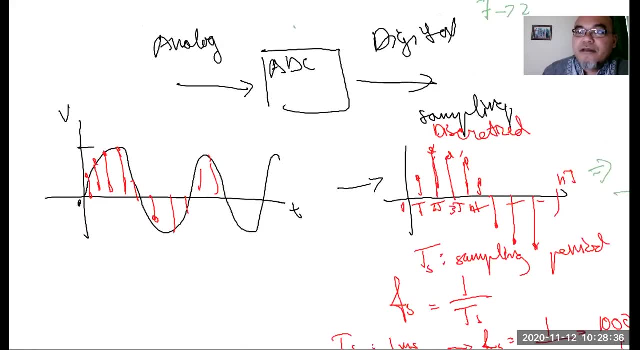 This in the bit it becomes because in computer we only work with one and zero. one and zero right. Seven is two to the power of equals to what Four plus two plus one right. So this become two to the power of two plus two to the power of one. 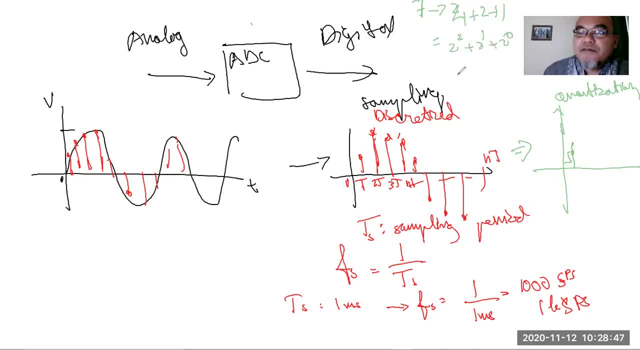 Okay, Okay, Two to the power of one, plus two to the power of zero. Or, if we express it in eight bit value, this becomes zero, zero, zero, zero, and then zero, one, one, one. Okay, So there are eight bit value. 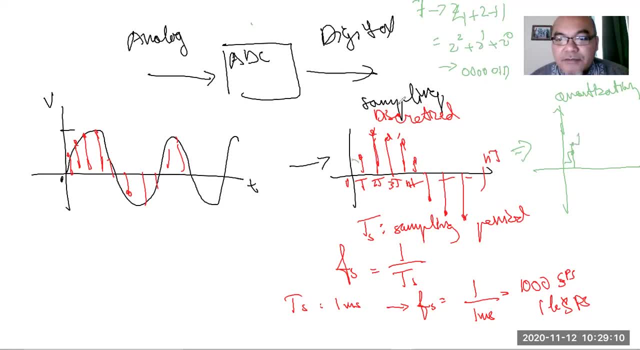 So similarly this one, the value here, will be quantized. So if we have eight bit, it means that a maximum eight bit is 238.. Okay, Roozbeh Gharakhloo, 256 to do the power of eight equals to 256. so we quantize this value into 256 level. 256 level, so if we have the full range is 10 volt, for example, the full scale rain is tenfold. it's each quantization level will be tenfold. if I did by 256. 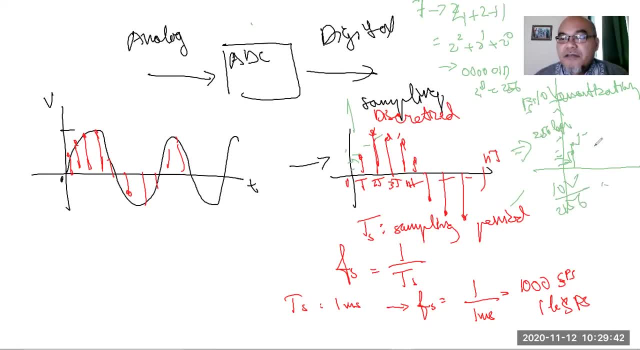 How many? so please calculate it. so we not only that the value in the digital signal will be discretized, like this, but it will also be quantized. so in, in, in, it will be in lock, like this, something like this: okay, so with analog digital conversion we lost the, we lost the signal in between. 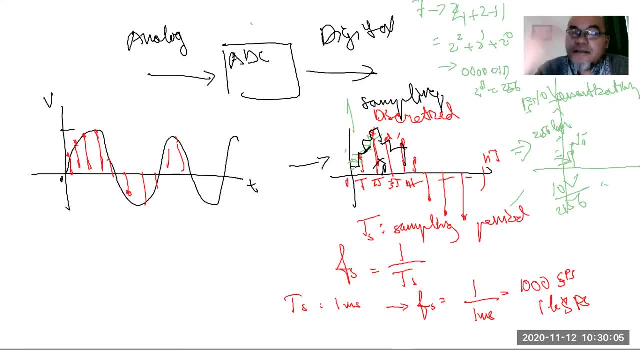 The sampling. so the signal here will be lost. and secondly, we will also lose the signal between The quantization. the signal in between we also lost, because it is being rounded it around it down, around it up. okay, so in another digital conversion. to summarize: there is discretization. 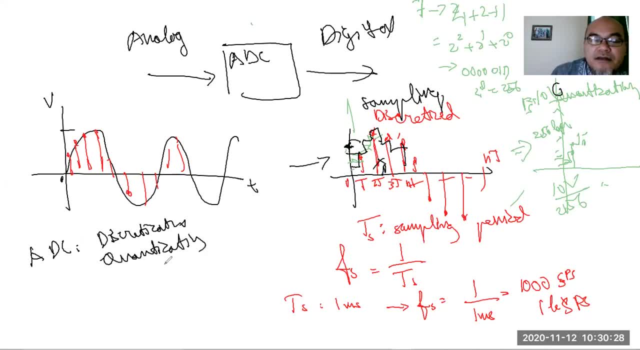 and quantization And in order that we can reconstruct the original signal from the digital signal- yeah, Usually. then the sampling frequency. here the sampling frequency has to be at least twice the maximum frequency of the bandwidth of that signal. for example, for ecg right the bandwidth is 100 hertz. if we want to be able to reconstruct the original analog ecg using our computer, then our sampling frequency in our adc have to be at least 200. 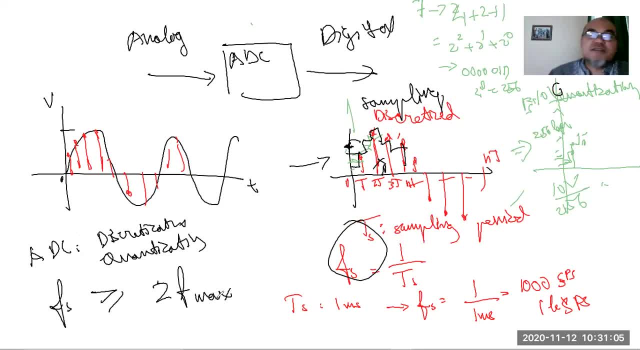 The more the better, the better. 400 it's better, 1000 even better. this is what We call as the night quiz sampling criteria. night quiz sampling criteria. This is in terms of sampling, That in terms of quantization. yeah, the more digit we have to quantize, the 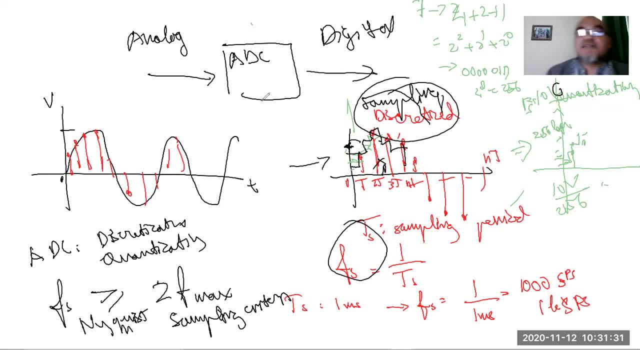 value of the analog signal. the higher the resolution, the resolution is better. so, for example, our full scale range is tenfold if we have only four beats. yeah, so the resolution will be then fall, divided by two, to the power of four. so tenfold divided by 16, how many is this? 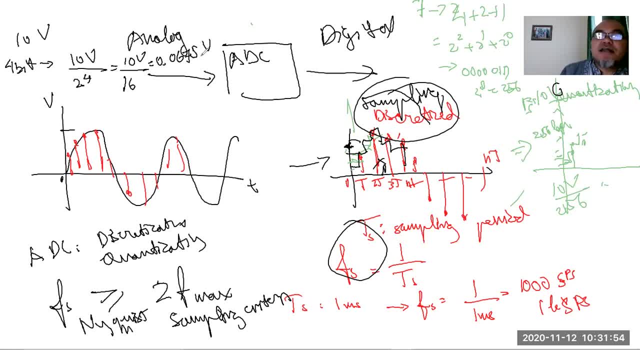 About 6.0675 fault, right. so each level in that four bit on Lincoln, only 0.0675 fault. so if you have a value of, let's say, 0.02 fault, it will be gone. 0.02 fault, it will be gone. 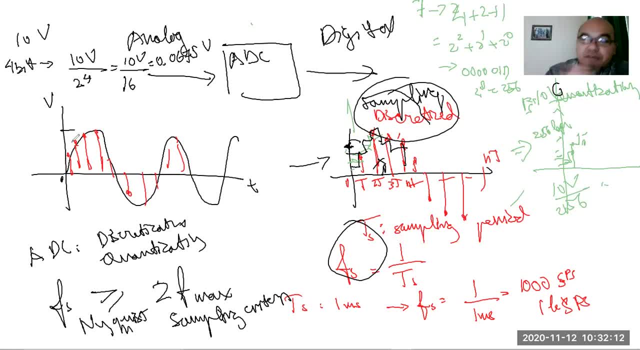 It will be rounded as zero. So what if we want to that, if we want to have less error, to do this rounding, do this quantization, then what we can do is increase the bit. the resolution of the adc So becomes, for example, it be it become a bit that the resolution will be tenfold divided by two to the power of eight, tenfold divided by 256. I don't know, I don't know. 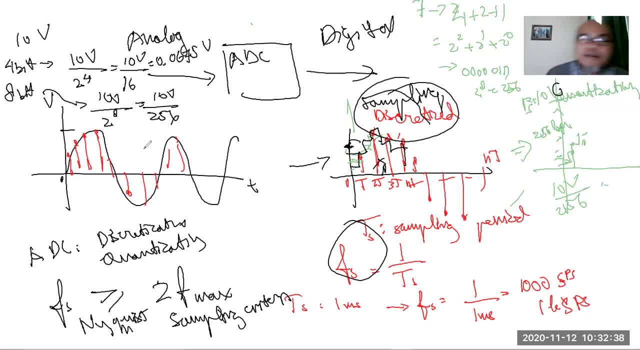 Ready with me if you can calculate? yeah, this can you. so this is Much. the value of this will be much smaller than this one. so it means you can quantize, you can approximate the value of the original analog signal better, So The filtering itself can be done at the analog level. we have what? 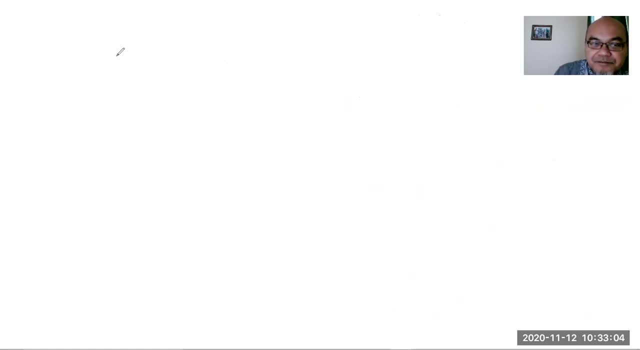 We call as No pass filter, so in low pass filter. So if this is the frequency domain And this is the signal the low pass filter will pass on, neither Low frequency from this cut off, what we call this cut off frequency, the frequency the signal having larger than this kind of frequency will be, will be filtered, will be stopped in high pass filter. in high pass filter it is the other way around. in high pass filter. signal with 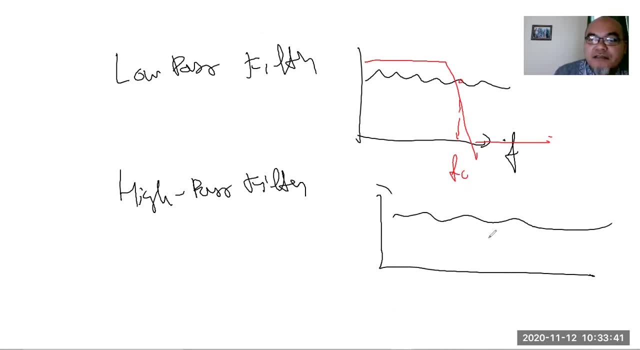 low cut off frequency. so if you actually get this, it will only pass The signal at this Frequency, larger than the low cutoff frequency. we have also what we call as Ben pass filter- Ben pass- What this been professor is. if we have the filtering is like this: so we have to cut off frequency.